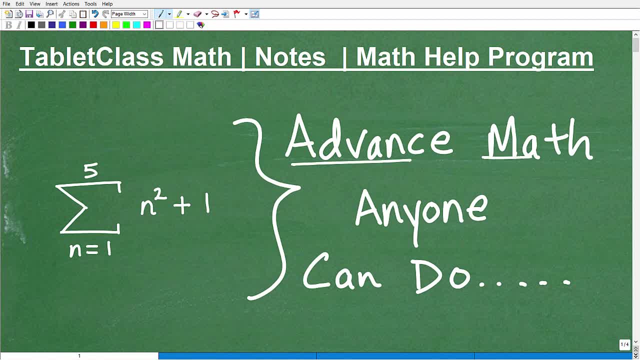 Okay, let's take a look at an advanced math problem. anyone can do So. this is the problem. We're going to do this in a second. And this word advanced is all relative. You know, what's advanced to you might be basic to me, And then there's levels of mathematics that I didn't take that are, you know, are very advanced to myself. I actually have a degree in mathematics. So, again, this word is a relative term, But oftentimes when we look at something, we look at it as a relative term. 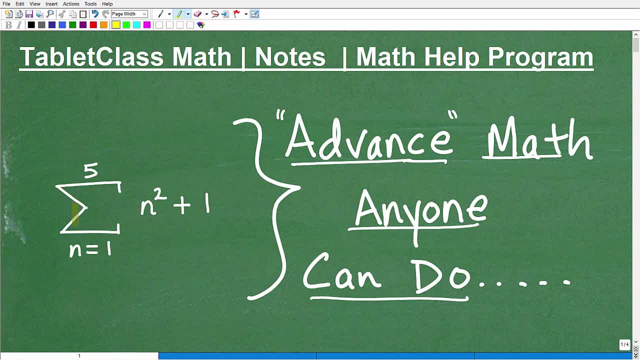 Something like this, something new. Okay, and I'm assuming maybe you've never seen this symbol before. This looks pretty intimidating, right, And it's like: what does this mean? You know, this is pretty scary looking, right. Maybe this thing has some teeth in it. you know, some sort of crazy eye looks, maybe like an alligator. What is going on? But oftentimes, I think a lot of students perceive math to be advanced because of the symbology the notation is. 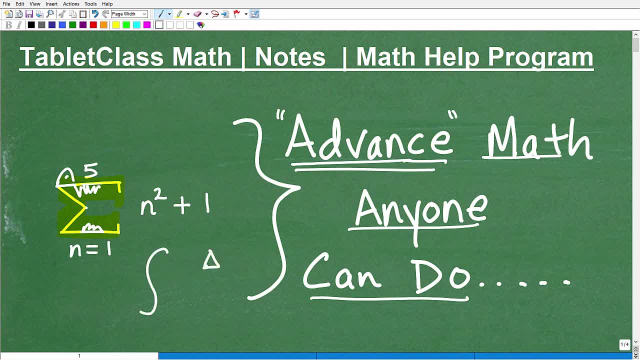 different. Okay, you have like crazy things like this or little symbols that you're not used to And you're like: what does that mean? That must be super advanced, it must be very difficult And in fact, you know some of these things are abstract in and of itself, But you know a lot of what you would perceive as being advanced math, and I'm talking about- probably for most of you out there- anything above and beyond algebra, maybe algebra to college, algebra, pre calculus, those type of things. 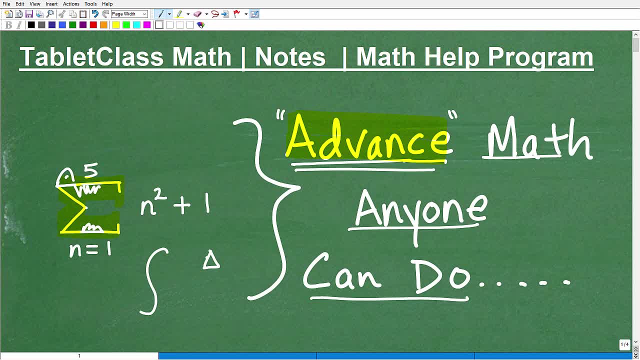 The notation that you're introduced to is new And I think that's can be a little intimidating. So my point here in this video is to show you that you know, don't be overly intimidated by advanced math. okay, you can learn it, But, like anything else, it's just learning one concept at a time. you kind of build yourself up And all these steps that you're you are learning are going to be applied in future topics that you need to learn: mathematics. 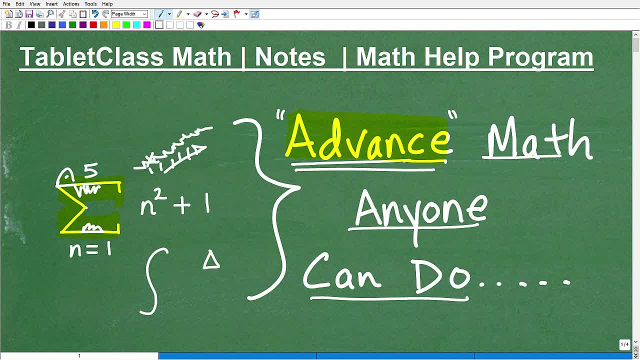 That's why it's important. math builds upon itself, And when you're not, you know paying attention or really you know building your foundation up. That's where I think people struggle in math, and now math becomes difficult. Okay, so we're gonna get into this problem in just a second, But first we're going to quickly introduce myself. My name is John. I'm the founder of tablet class math. I'm also a middle and high school math teacher And over many years, I've constructed what I like to believe is one of the best online math video programs there is. Of course, I'll let you be the judge of that. You can. 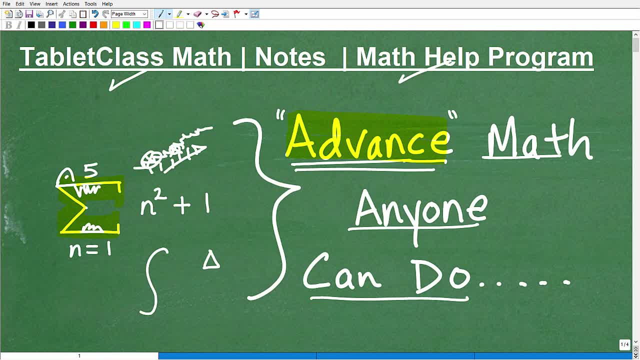 find a link to it in the description of this video. But my math help program. I have full math courses. So if you need to take a full, complete math course, I can help you out, And if you need assistance in your current math class, I can help you out. So I offer full, comprehensive, very in depth, full video lessons and I teach you how to solve the most common math problems you know that you're going to face as a middle and high school math student, and even in college. So I do thousands of problems. It's taken me years to 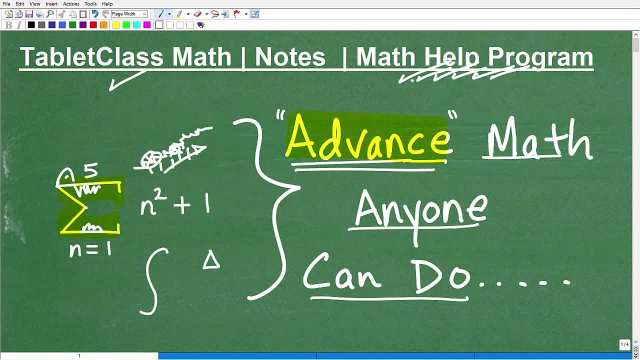 build. So again, if you're interested, you can find the link in this video. Now let's talk about notes. I'm going to make an assumption that you're probably taking some sort of math class right now, Or maybe you're planning on taking a math class. The thing that I like to stress about notes is this: over decades of teaching math, it's apparent to me that those students who take the best math notes almost always have the best math grades, and the reverse is true. If you're not taking good math notes or you 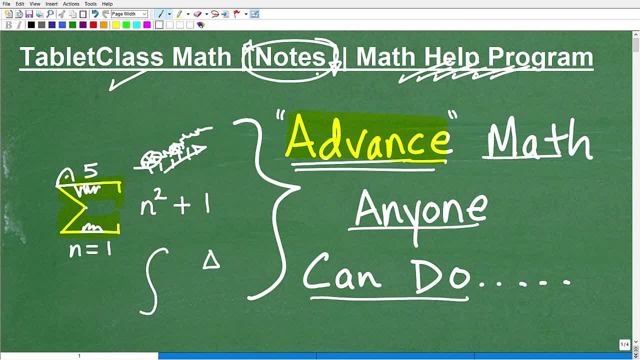 have sloppy math notes or inconsistent math notes, then math is going to become difficult for you, Okay, especially here in advanced math, it's becomes even more critical. Okay, so, as you progress in your mathematics journey, you have to be a great note taker, but it's a skill you need to take on to improve. take a look at where you stand and improve if you need to improve. But in the meantime, if you need something to study from, I actually offer math notes. those will include pre algebra. 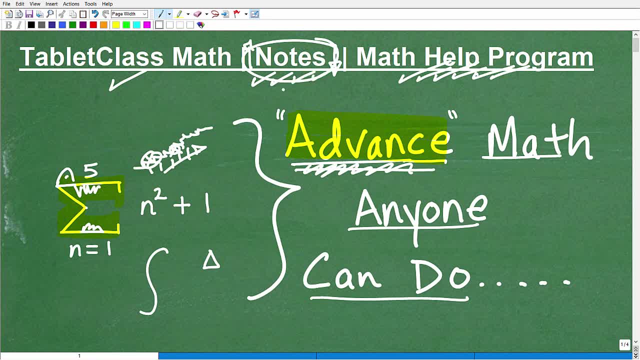 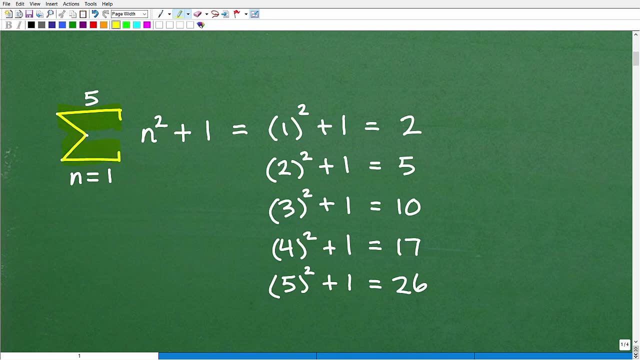 algebra one, geometry, algebra two and trigonometry. you can find links to those in the description of this video as well. Okay, let's get into this advanced math problem that anyone can do, Alright, so here it is, this little thing here. okay, this is what we call a sigma notation. sigma like this: it's a Greek alphabet type of deal, And this symbol like this basically means: 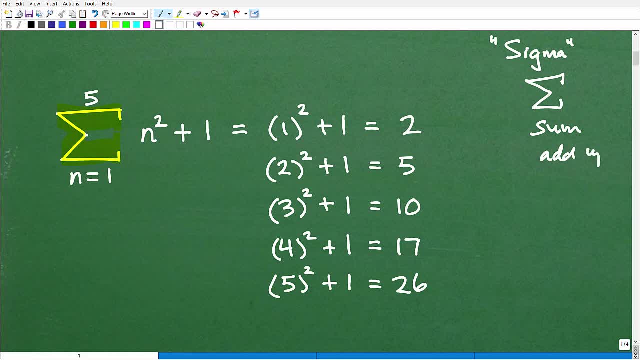 sum, okay, just means add up. add up, that's all it means. Okay, so you know the symbol is telling us to do something. okay, your means, you know, add something up, And this has to do with the more advanced math concepts called sequence and series. All right, And a sequence, just real quick would be something like this one: No, let's say three, five, seven. you can see a pattern going on here. right, So this is a mathematical sequence. 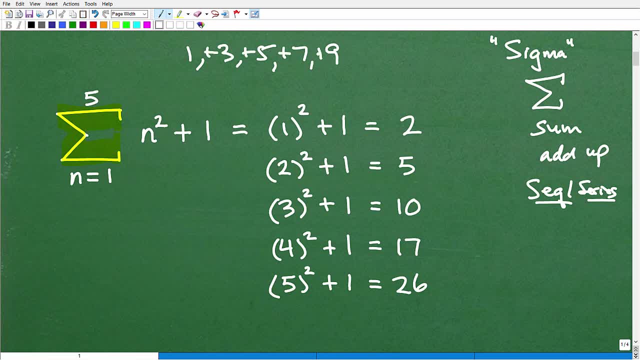 And if I was to add all these little terms up here, we have a series- And this does relate to more advanced mathematics in terms of it's kind of getting ready for you to study calculus. okay, because we have another symbol, like the sigma symbol. to sum up, in calculus it's called an elongated S. you've probably seen it looks something like that, looks kind of crazy, But these symbols mean something, right, And it doesn't have to be, you know, a series. 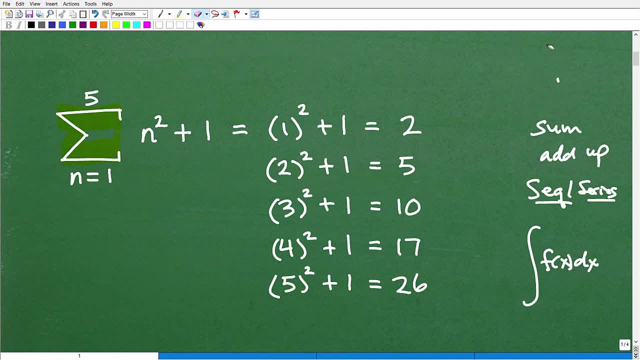 overly complex. anyone can understand this. so let me go ahead and show you what's going on here, and then we'll go ahead and wrap up this video. all right, so what this symbol is telling us is to we want to take this little thing right here, this n squared plus uh one. let's do it over here, and 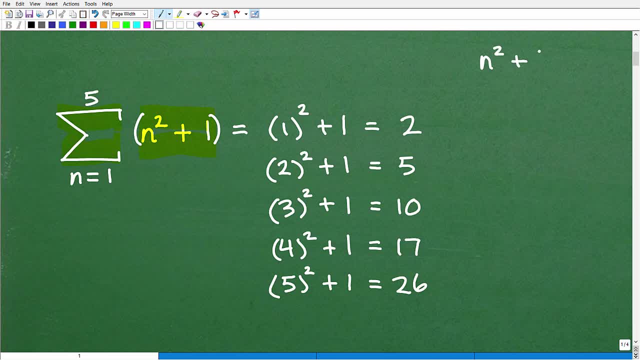 we see i already have some work done. let's just pay attention real quick over here. n squared plus one. okay, n is just a variable. okay that we could plug in any number to. okay, when we plug a number to uh n, it this thing becomes a value in and of itself. okay, so i plug. 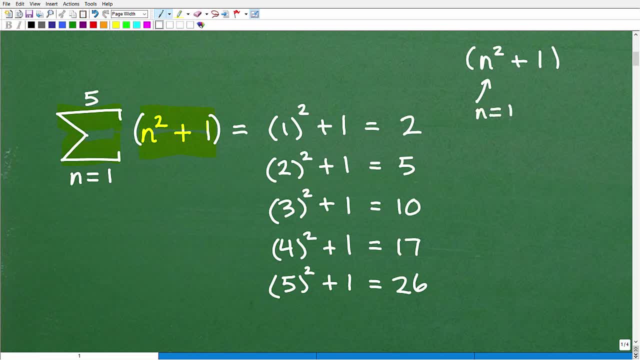 in n equals one. right, if i let uh n equals one and i plug it into this n squared plus one, that means i'm going to go: okay, i'm going to plug in one for this n and i'm going to square it plus one. one squared is one times. 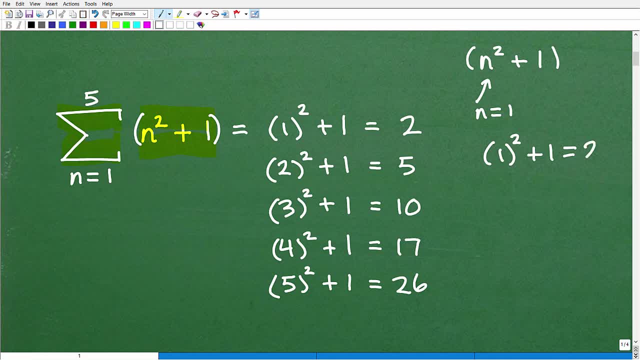 one squared is one times one, one, which, of course, is one. one plus one is two. all right, so what we're saying here with this symbol is telling us to do, is saying: okay, i want you to, uh, start from one, start from one and go all the way up to five. so we're going to go from one, two, three, four and then we'll stop at five. 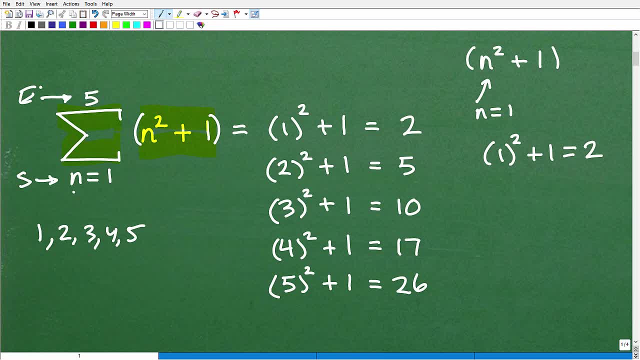 so this is the starting point, this is the ending point. okay, or the starting value and the ending value, and when we do something called indexing, we're just going to start there, we're going to move up. okay, we'll keep going all the way to five and we're going to plug in these respective numbers. 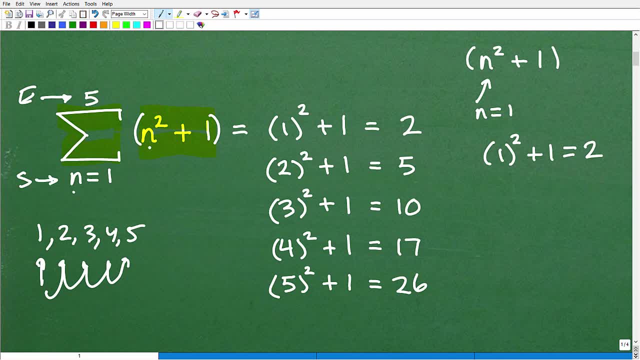 okay, into this, into this little expression, this algebraic expression here, and then we're just going to add up the results. that's all we're going to do. okay, so we'll start with n equals one. there we go. so one squared plus one is two. okay, we're done with that. now we'll move on to two. 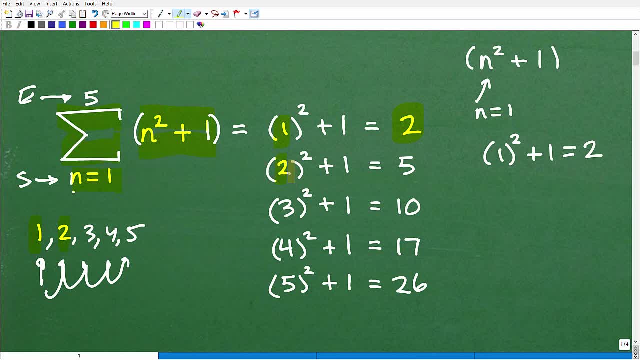 okay, so two. we're going to let n equals two. all right, we're indexing up. so that's two squared, which is two times two, is four plus one is five. okay, now we'll move on to three. so three squared is nine, okay. or three times three plus one is ten, okay, now move on to four. so four squared is 16. 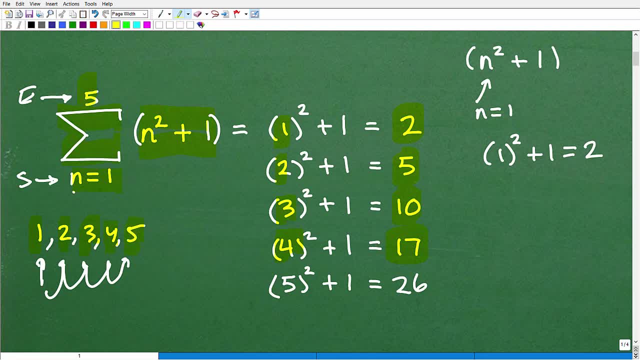 plus one is 17, then we'll we'll finish up at five. so five squared is 25 plus one is 26. okay, so what we want to do now is add all these guys up. so the way you can- another way you can kind of see this is this way. okay, so this is what this means. all right, we're going to start with one. 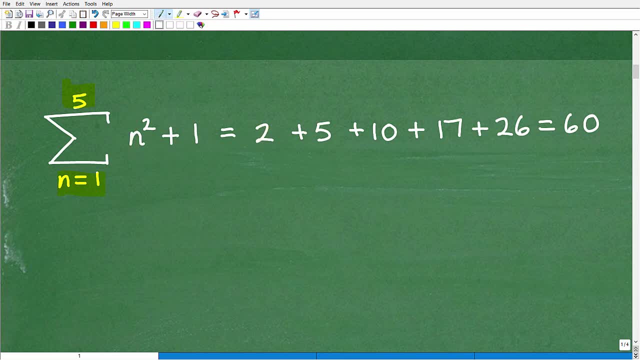 and at five, n squared plus one. so this is where n was equal to one. this is where n was equal to two. this is where n was equal to three and is equal to four. then we'll stop here. n is equal to five and we have these respective terms here. okay, of this series, and now i can just add all these guys. 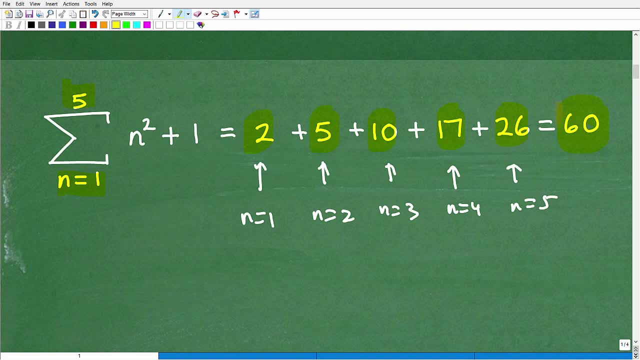 up, two plus five plus 10 plus 17 plus 26 is 60, okay, so this symbol, okay, is a convenient way to express sums, okay, sums of what we call a series and and you know. but you can have all kinds of various patterns and ways to get. 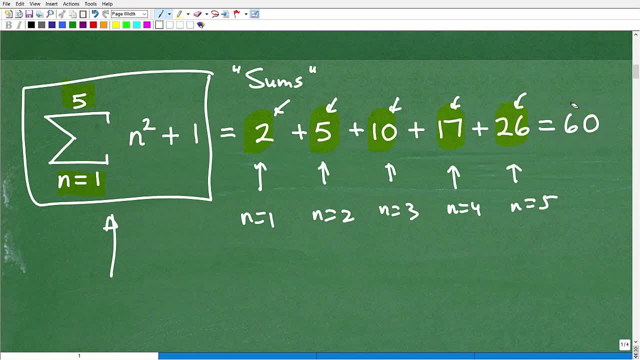 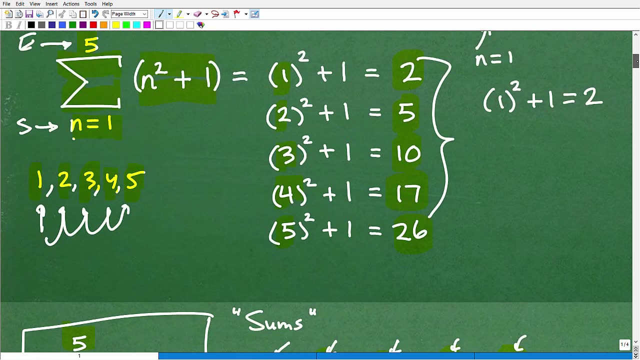 these terms okay, but in mathematics, what we'd like to do is to use short cut notation, okay, notation that we can understand what's going on, to make our life easier. okay, and a big part of advanced math is understanding that notation. remember, math is a language and it doesn't have 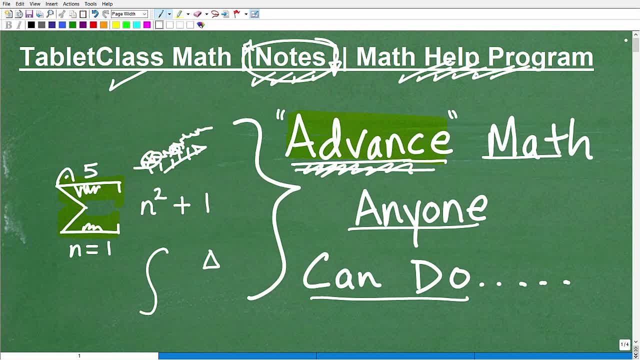 to be that difficult. okay, again, i think, where math becomes difficult for a lot of people. i'm not saying that there's not abstract concepts in mathematics. there definitely is okay, but i think more often than not, the challenge for a lot of math students is they- uh, they're not focused enough. 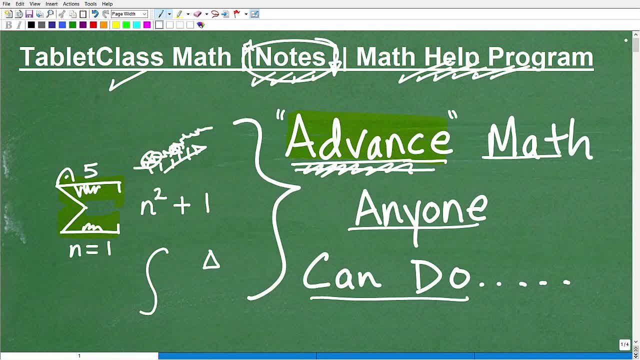 on building up their foundation. okay, you got to pay attention in math. it's, you know, it's very much like driving a car, okay. so here's the road, here's your car. okay, just because you've been keeping your car, you know in, you know the lane. okay, you're keeping yourself off the side of the road here. 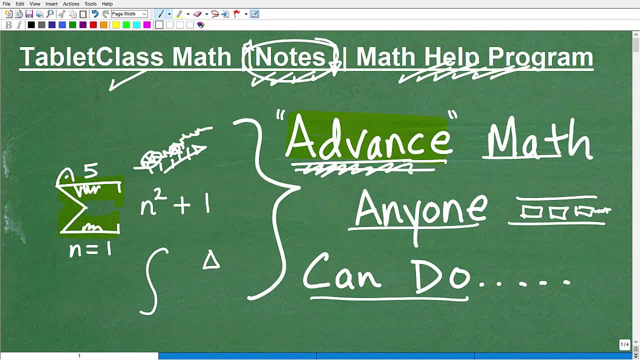 you have to always pay attention to keep yourself on the right path. and the same thing in math. okay, as soon as you take your eye off the road, think bad things can happen. and in math, uh, you know, as soon as you stop paying attention, you're like: oh, i've been doing good, i've been doing good, you know, just for the last. 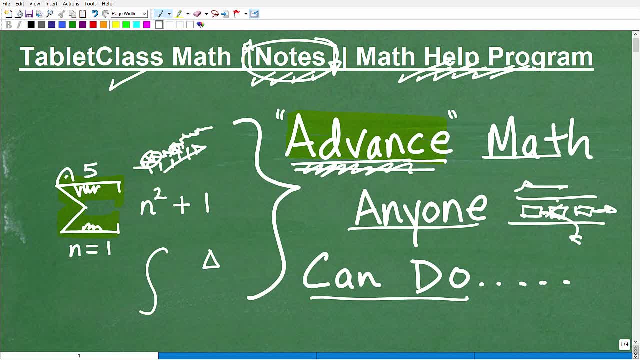 300 miles we've been driving safely. that has nothing to do with the next mile that you're going to drive, right? if you stop paying attention immediately, things can go wrong. same thing in math, okay, especially in more advanced levels. you have to always pay attention and be focused. all right, 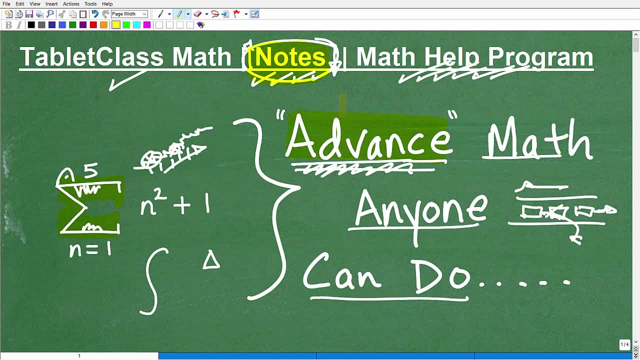 note-taking is so critical um having strong math notes. believe me when i say these things, i'm speaking from years, decades of experience. okay, all right. so if some way you like this video, we're entertained by it, enjoyed in some manner, please consider smashing that like button. and if